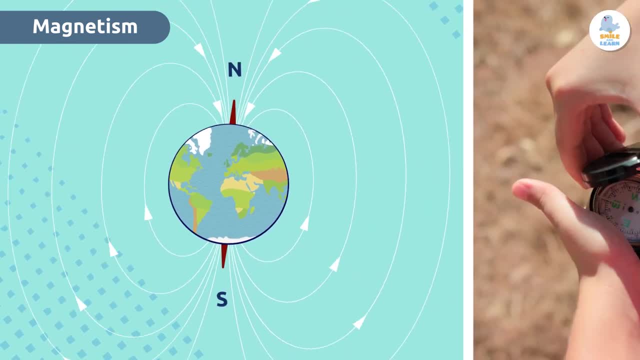 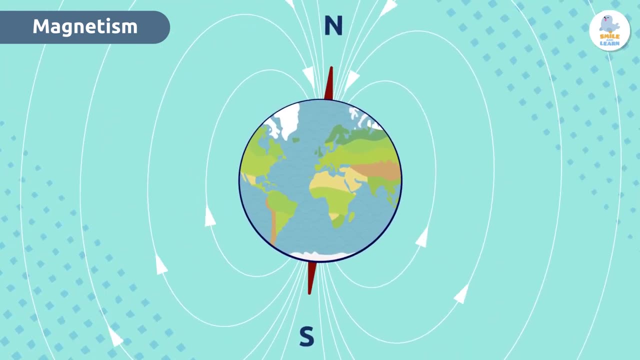 a magnetized needle that always points to the Earth's magnetic North Pole, which allows us to locate ourselves on a map. And do you remember what a magnetic field is? Yuck, Exactly, It is the space surrounding a magnetic field where particles throw were made. So you've. 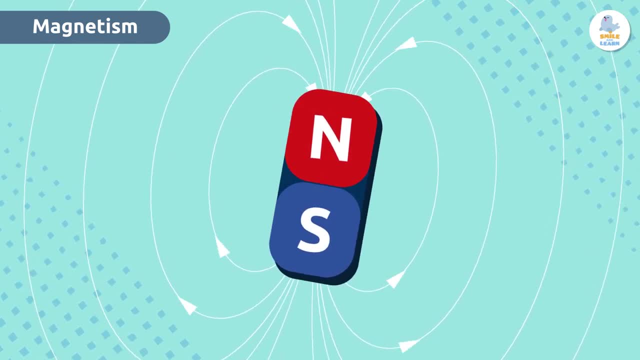 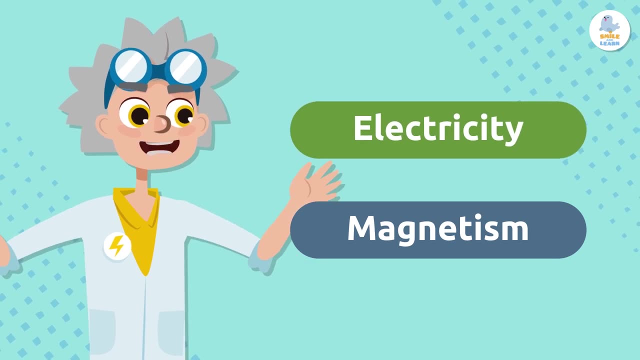 got the first magnet of the Universe. Okay then, how would you estimate the magnetic? a magnet where its magnetic force acts. In other words, it is the space where a magnet can attract other metals. Now we are ready to learn what electromagnetism is. Here we go. 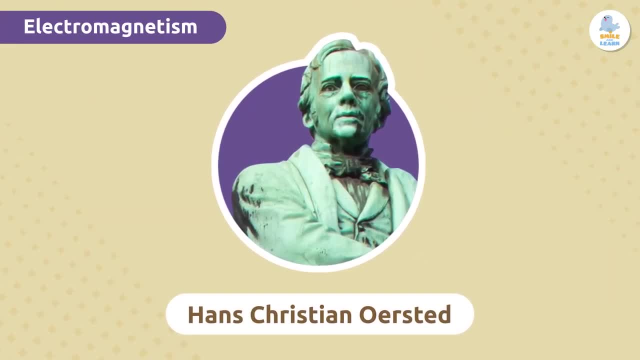 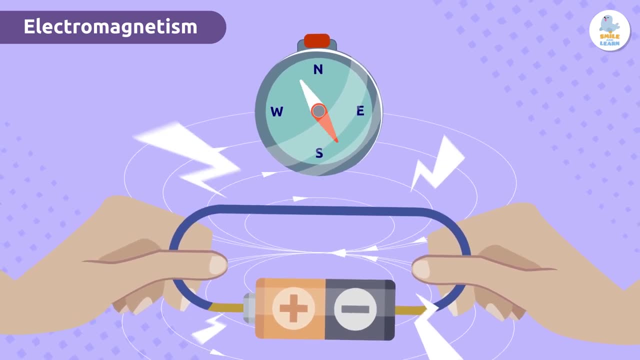 Let's start with a bit of history. In the 19th century, a scientist named Hans Christian Ørsted discovered that when he brought a compass close to an electric charge, the compass needle didn't point north anymore. What do you think this meant? 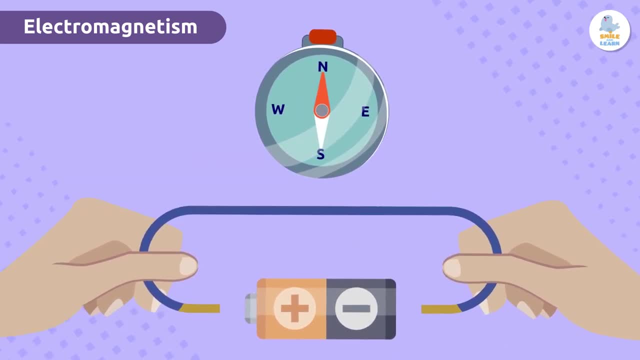 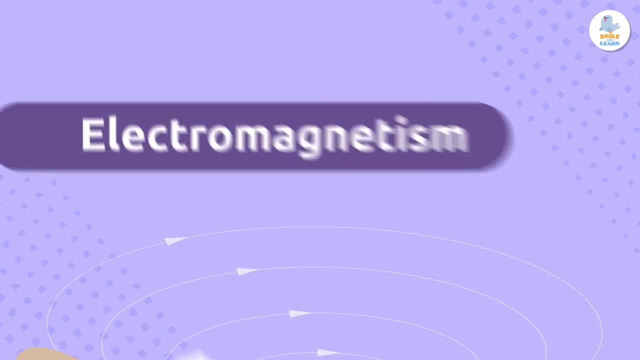 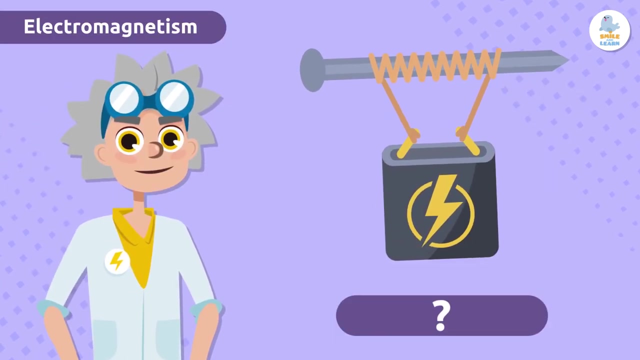 That's right. electric currents produce a magnetic field. Wow, We call this relationship between electricity and magnetism electromagnetism. Let's see if you can guess what this is. It's an electromagnet. We can generate a magnetic field very easily thanks to electromagnetism. 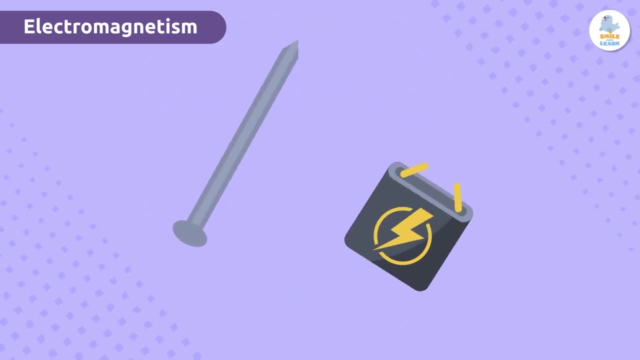 Let's see if you can guess what this is. It's an electromagnet. We can generate a magnetic field very easily thanks to electromagnetism- electromagnets- This involves tuning a metal bar into a magnet by connecting it to an electric current, in this case a battery. To do this, we wind a wire of conductive material, such 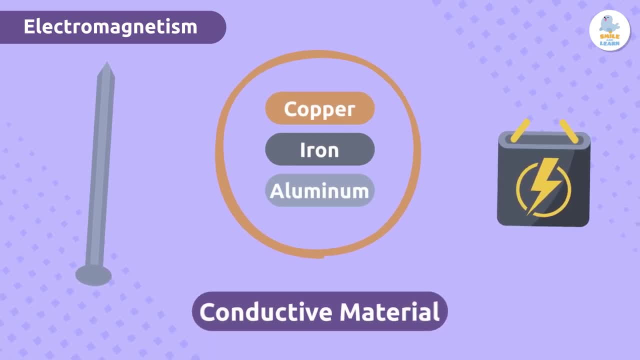 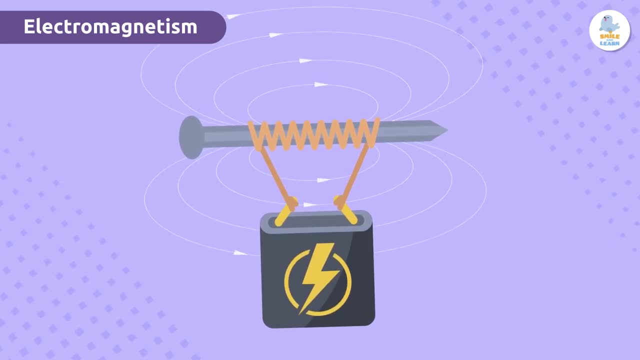 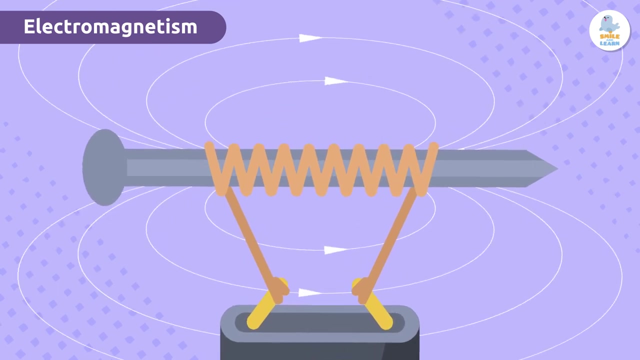 as copper, iron or aluminum around the metal bar. So why are we doing this? Remember how I told you earlier that electric currents generate magnetic fields. Well, this wire's magnetic field is very weak on its own, So by wrapping it around the metal bar in a spiral shape, we concentrate the magnetic field in a small 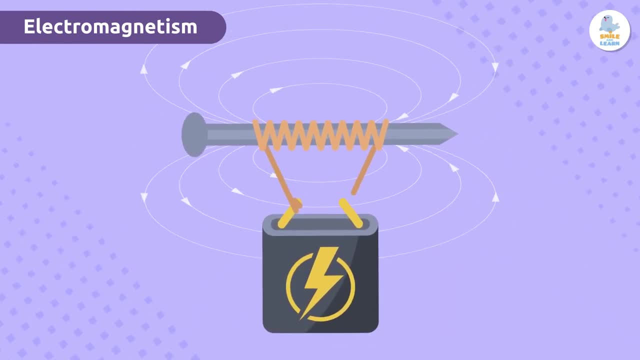 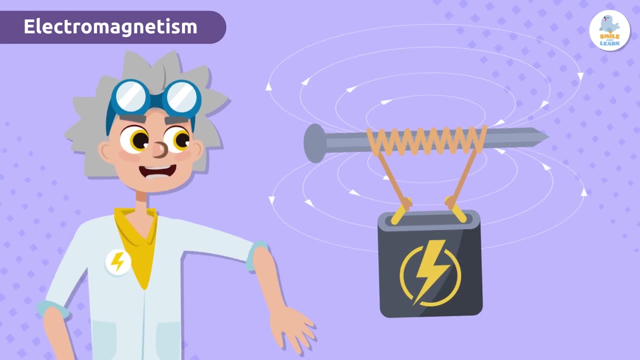 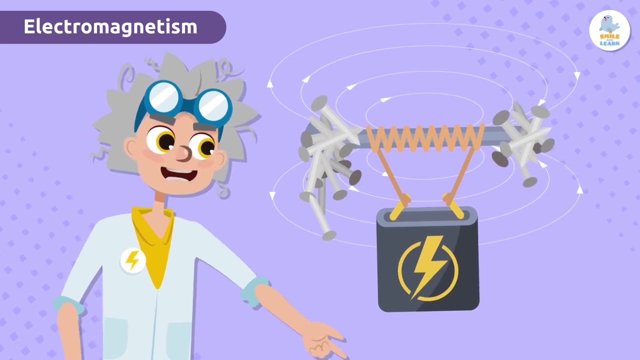 area, which increases its power. When we turn on the electromagnet, the electric current starts to circulate, activating the magnetic field and attracting nearby metals. It's impressive, isn't it? We can also use electric electromagnets in a variety of ways. We can find them in bells or car brakes, but we can